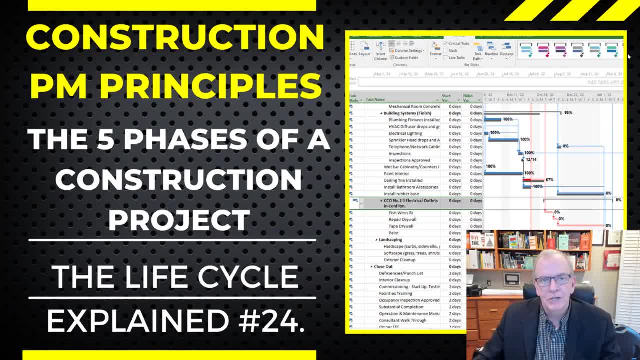 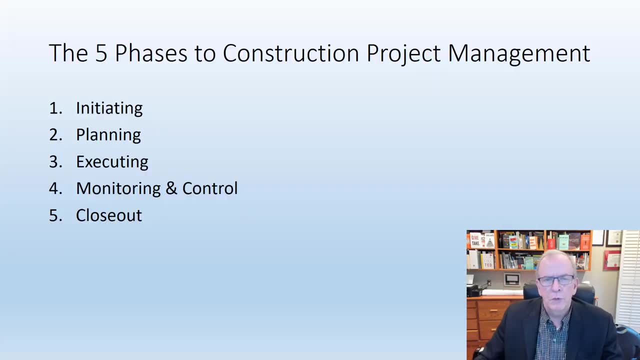 Hi, I'm Tom Stevenson and welcome to Construction Project Management Principles. Today we're going to be talking about the five phases of a construction project, What's involved in the life cycle of a typical construction project. So when we think about the five phases of a 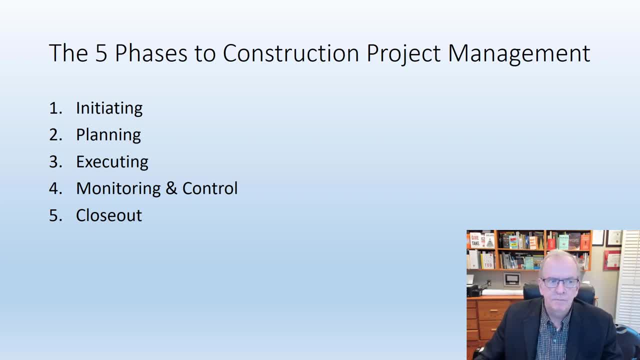 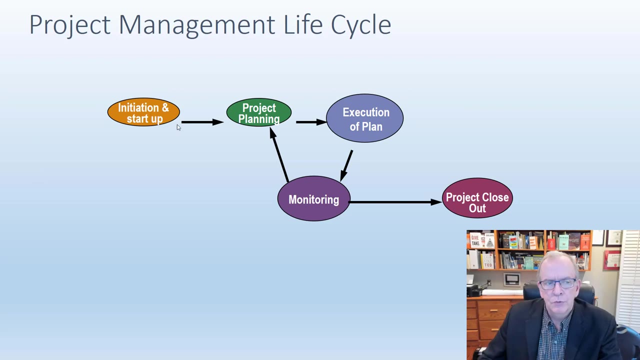 construction project. we have initiating, planning, executing, monitoring and control and close out. These are the five phases and if we want to sort of look at it in a graphical form, we can think about it this way: We start the project, we have initiation, we've won the project. 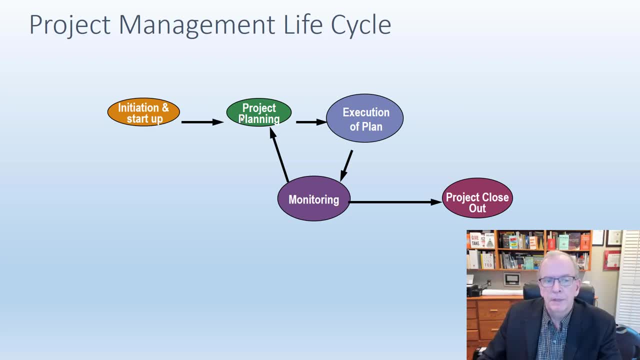 and we're going to be starting it up. We have project planning. that's the phase where we're planning what we're going to do and how we're going to do it. Hopefully we do that pretty well. Then we're going to execute the plan, So we're actually running the project we can imaging. 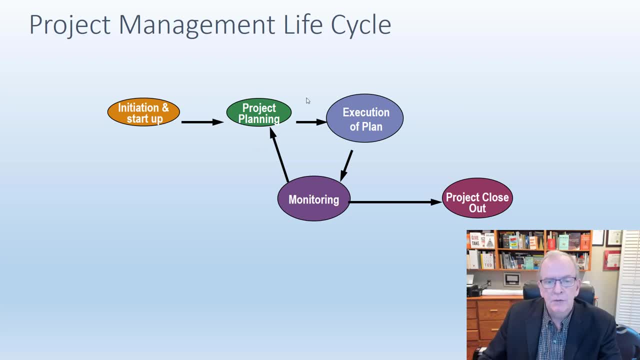 monitoring the project And you'll see in a minute how these four here interact. And these should all be leading to project closeout. So let's start at the beginning. here We have pre-construction. We call that early phase, before you're actually starting to excavate in the ground, get things delivered and installed. We call that all pre-construction. 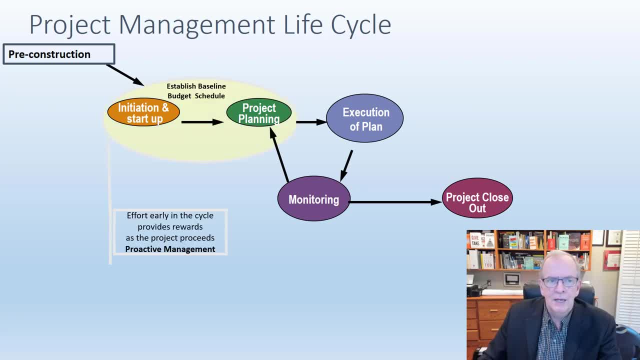 So hence we have pre-construction planning And in that planning phase we are establishing a baseline for our schedule and a budget. right. So we get a baseline schedule and a budget schedule. We have two things that we are doing: the baseline for the budget and the schedule. That's so that we can measure and compare. So we have a plan and we'll be able to measure what the plan was as things change. 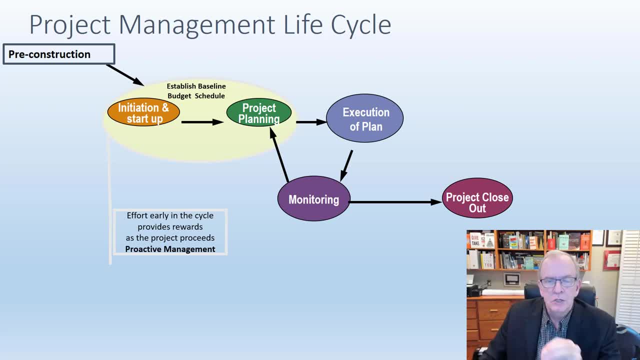 And, believe me, in the world of construction things change. Nothing ever goes exactly to plan, But that's okay. That is why we do this process this way. So we start out and if we put in good effort early in the cycle, we get a lot of rewards later on. We call that proactive management, where you're actively looking ahead. You're not waiting for things to happen to you. You're planning ahead so you can make things happen. 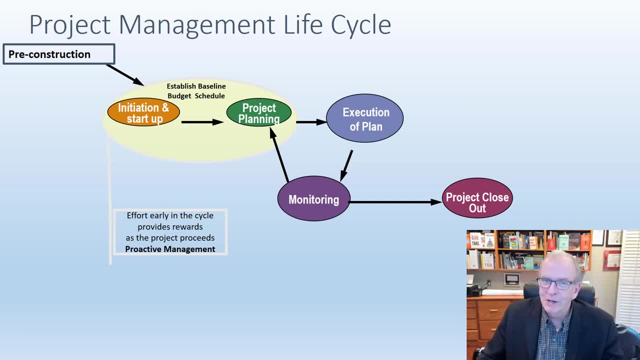 And that's very good. But we are under a lot of incentive in construction to actually just start and show things that we're doing. But that doesn't help if we have to redo things. So we want to be very cognizant of that. 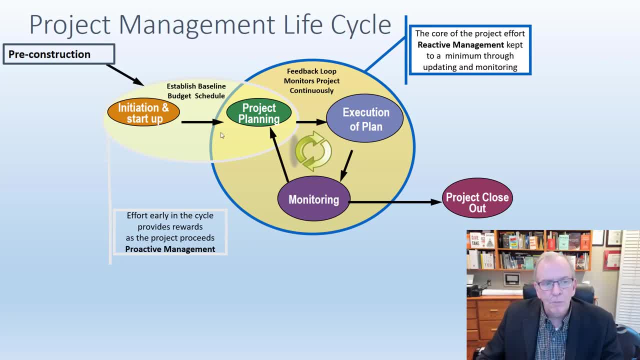 We start the project. So we planned it. We've got it all planned out. We've figured out- you know the schedule, step by step- what we want to do, how we want to do it, We budget it, And the budget comes from the estimate that you made. 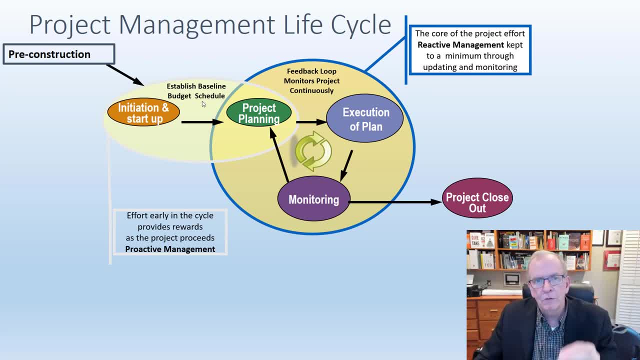 It allowed you to get the project. So you're breaking that up into various costs so that you can check how you're doing as you proceed compared to the baseline. So then you're starting the project And it should be this feedback loop Because, as I said, nothing goes the way you planned. Planning is a dynamic item, So this is not linear. That's what everybody thinks It's linear, But it's more iterative, back and forth. 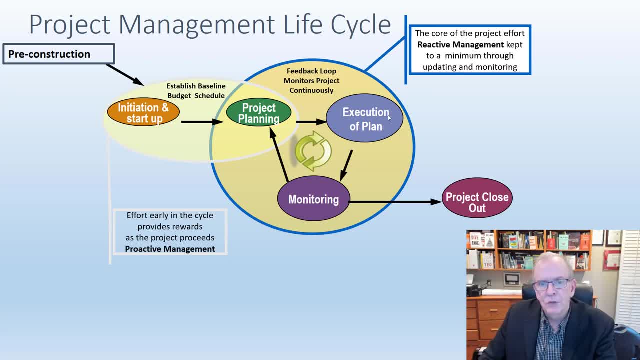 So we're planning, We're executing the plan. execution of the plan. We're implementing it And we should be seeing: how are we doing? There's this rotating circle that occurs here. How are we doing? And that's what the monitoring is. It's checking. 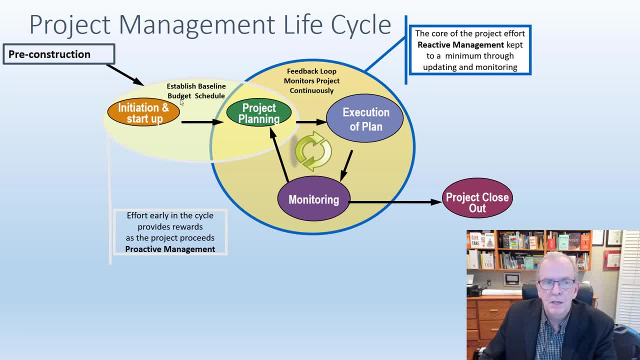 how are we doing compared to our baseline budget and our baseline schedule? Is there something we can learn from this? And the better we are at this, the quicker we're learning? There's traditional ways that we do things in construction And a lot of those traditional ways they're giving way to. 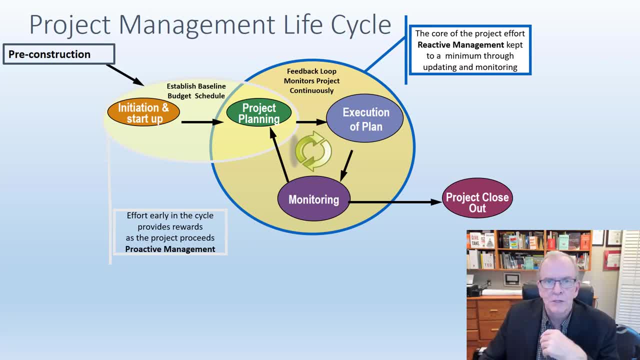 other ways of doing things or combining with other ways of doing things. So with the baseline schedule, that's great. We develop what we call a critical path, the steps of how we're going to do the project. But we've got to find ways that we get feedback quickly so we can pivot, we can adjust. 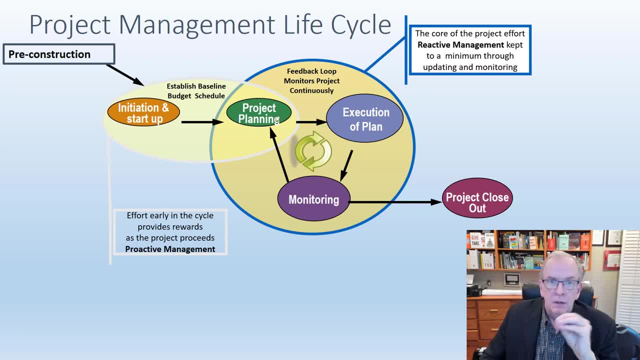 we can iterate and replan. Something delays us. we've got to adjust it. Maybe we still want to finish on time. Maybe we still want to finish on time. Maybe we still want to finish on time the same date. We've got to adjust our schedule going forward. So these are things that continuously 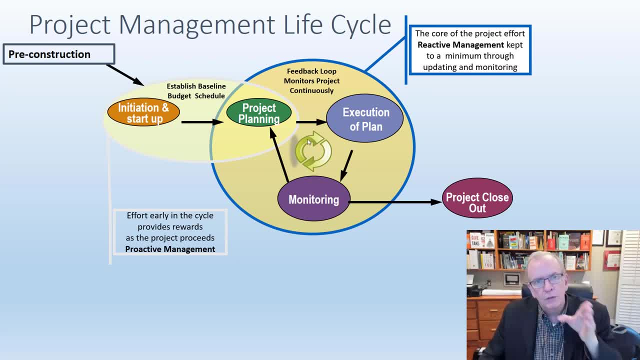 goes round and round here as you are building the project. So this is this cycle that's continuously rotating. We did something we planned out the week ahead. we check daily to see how we're doing. we're adjusting As we move through this. we're going to be headed towards the last stage of 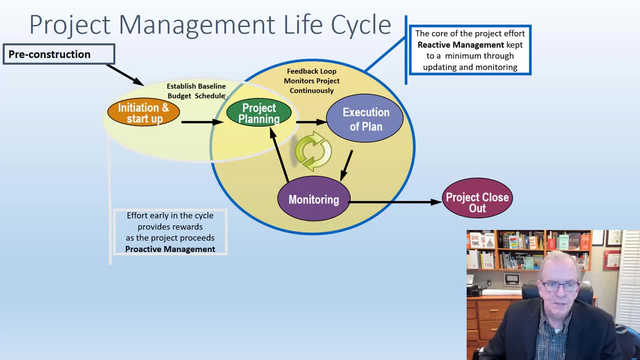 project closeout. Now, what I didn't say is that in the planning process we should be planning how to close out the project. We don't wait till we get here to start figuring out how we're going to close out the project. We started here And that means we fix as many deficiencies as possible. 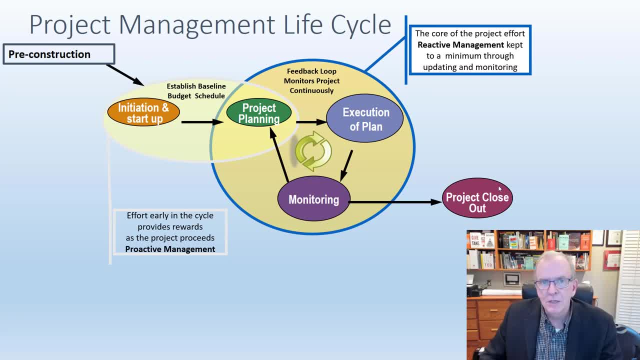 in this cycle. We don't wait and have a gazillion deficiencies, also known as a punch list, that we have to deal with at the end of the project. We're proactively planning, We're not getting here and then reactively responding to all the mess that we created. 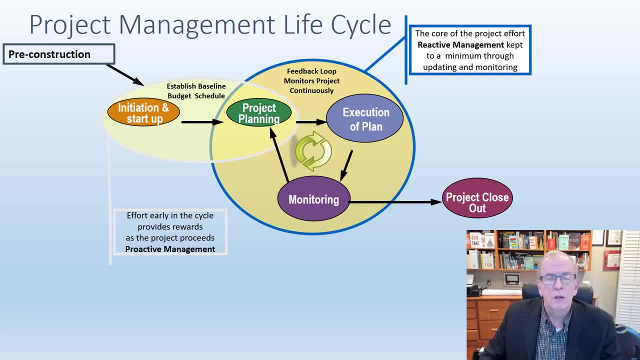 In the project planning process we also plan out commissioning. Commissioning is the testing of all of the building systems to make sure that they're functioning the way that they were designed to function. Very often there might be a third-party commissioning agent for larger projects. 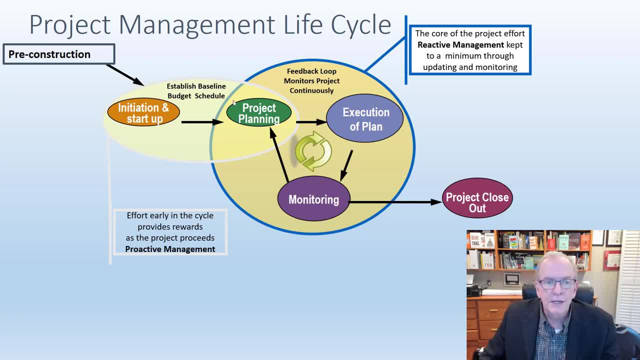 that the client has, and they're going to be checking things, But you want to find out exactly what their expectations are, And that's what we're doing, So we're not getting here and then reactively которой septic f? Tirưng Action. 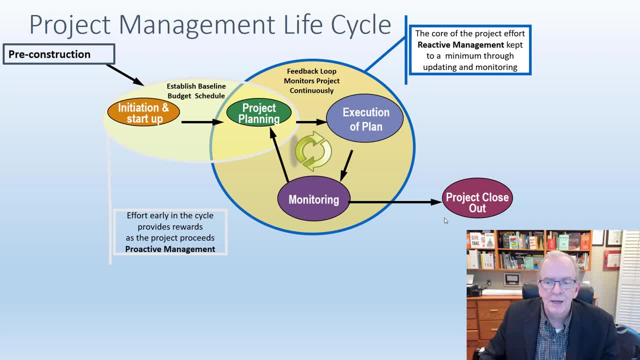 cher kwi ankles. So what happens when you get there? You're able to get here. It doesn't impact your type of window section. so your fully open backpacks will be a little moreyen. As I say, pics at the end are fun. 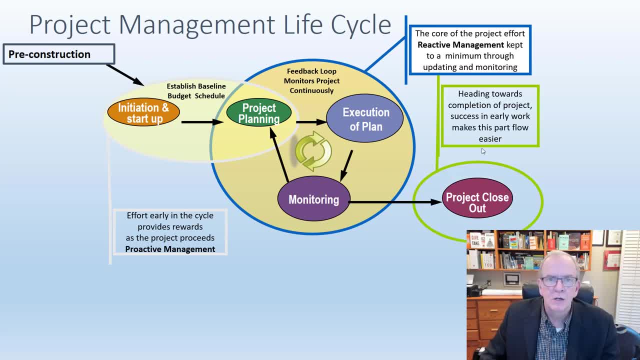 When you get at a interval in that area- If I get till here- it actually becomes much easier to close out the project. The closing of the project should take like around 10% of your time and effort. It shouldn't be like 30% of your time and effort. The big question is: time and effort are coming through. 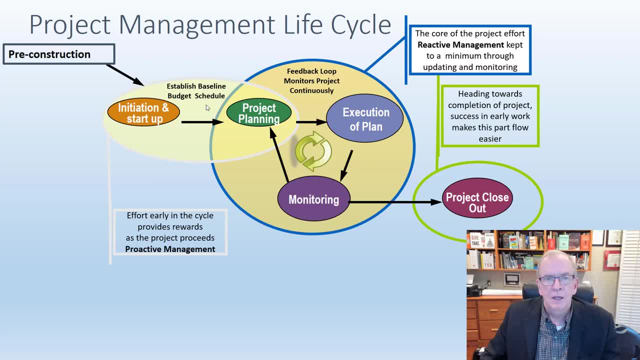 here. As I said, your planning cycle is very important too And, as I said, it is a dynamic cycle, So it's ongoing. so it's ongoing and iterative. Now, if we do this, we're really reducing the amount of reactive. 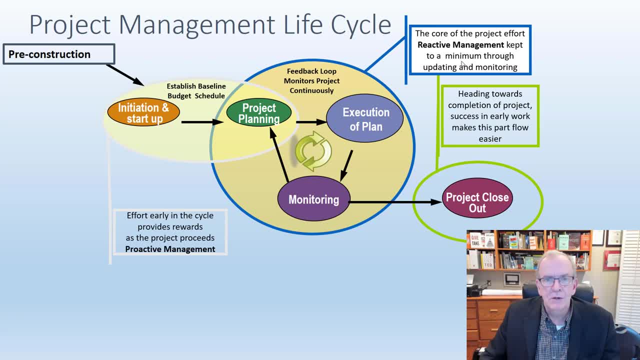 management that we have to do Now. I'm not going to say that you're not going to have to react to things. Construction is a very complex industry. our buildings are very complex and there's always things that are going to happen that you didn't expect, like black swan events. unknown, unknowns. 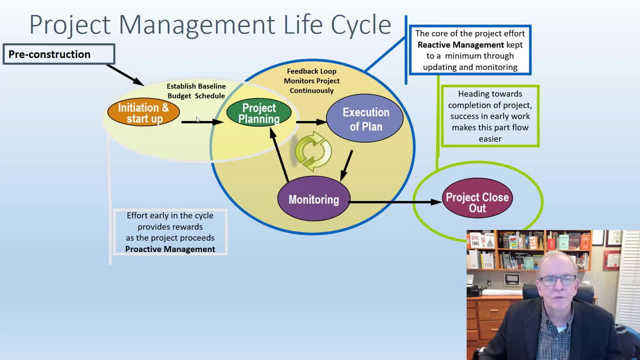 But we don't want to be reacting to things that we should have saw coming. we should have had contingencies for so that we can adjust when they happen. we've already got something that we can deal with it, Because when you are in reactive mode, you don't have time to re-plan the work. 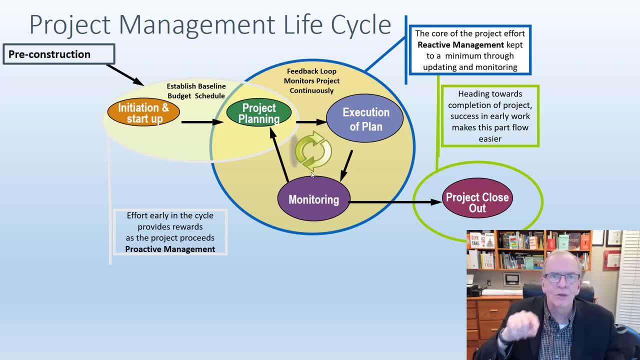 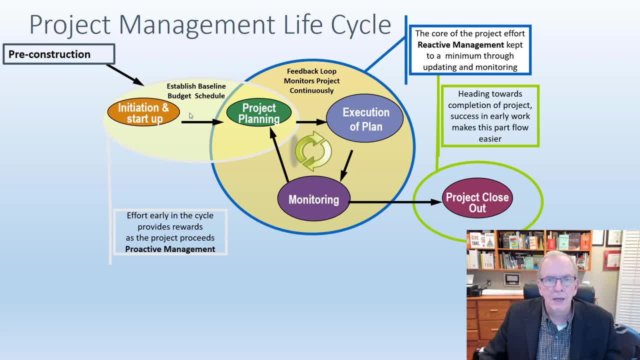 many times over. but we can compare to our baseline and see how we're doing and if we're documenting it well, we can learn going forward in future projects. So if we do that- and we do that with continuous communication with each other, between the GC, the consultants, the trade- 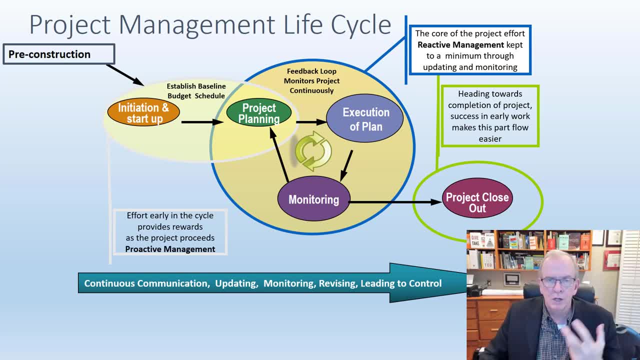 partners, the authorities having jurisdiction and, of course, the client. that will be very helpful for us and our success, especially if we do it in a way that we engage them throughout the project, Updating and monitoring. So we have to update to see where we are Monitoring. 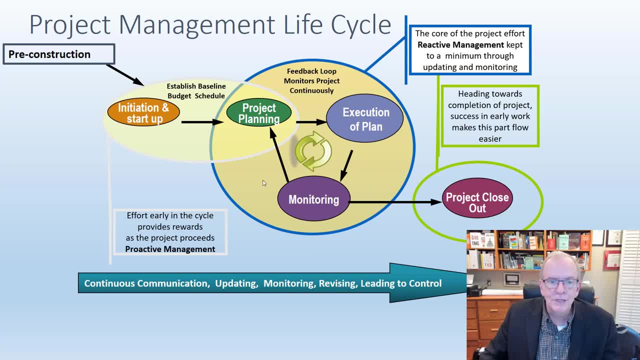 revising. so we have revisions and recoveries that we're doing in here and with the re-planning of the work. so once we have it updated, then we're re-planning the work, we're doing revisions and recoveries to get us back on track. that's going to lead to control. that's going to lead to success. 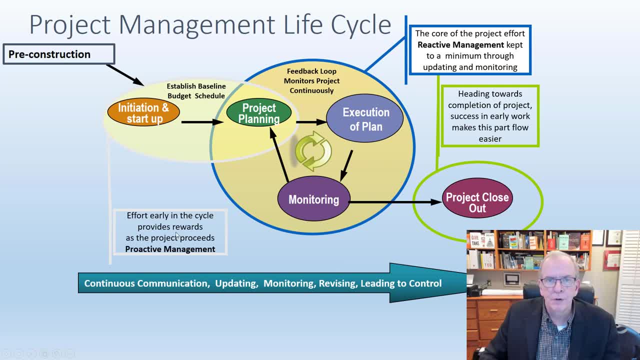 So this is the five stages of the project management life cycle, and if we do all of these things well, it's going to be very helpful. I have just a couple of other points that I'm going to add to this, because this is something I'll talk about in some. 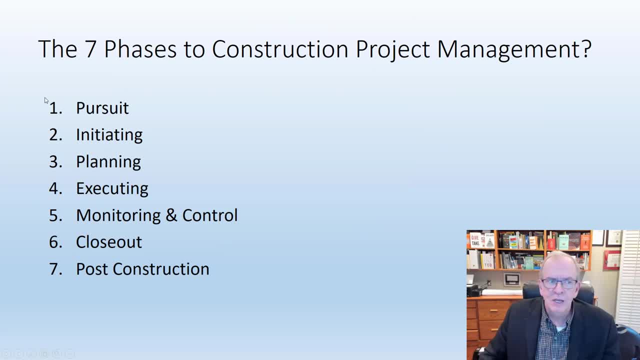 other videos. It really is seven phases when you think about it. Number one is: well, we've got to get the project. So there really is an earlier phase to this. but often we don't get past this phase because we don't get awarded the project, our price is too high or something's not standing. 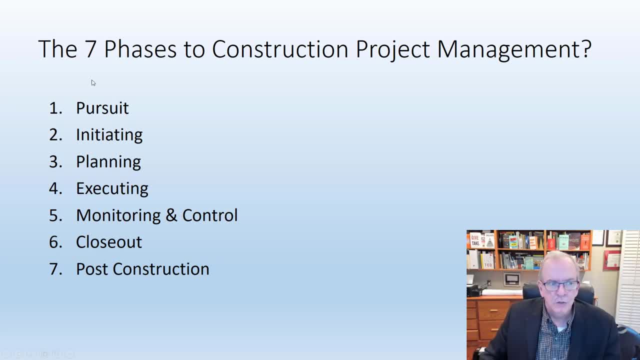 up to the RFP price. So we're going to have to get the project done and then we're going to have to P points process. so we might not get that, But when we do then it's going to lead to the other. 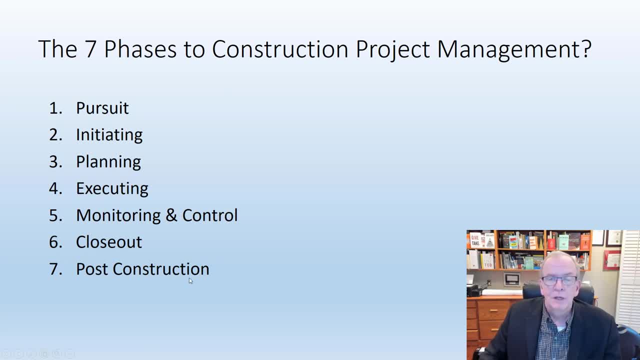 five. and then if we do the other five really good, you know what? then? post-construction services: there might be maintenance contracts that you can get out of this. you might have client. that client might want more work. you might not have so much difficulty getting the next project because